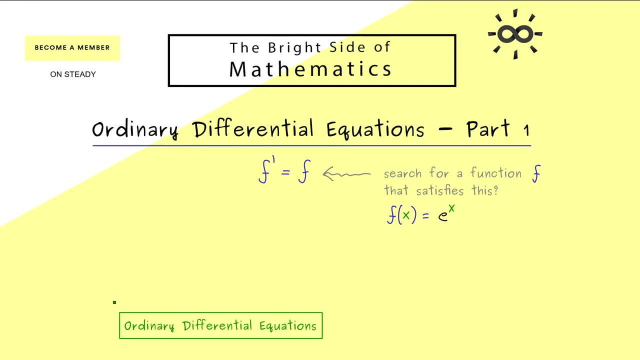 the description. Okay, now let's talk about the requirement, the knowledge you need to understand ordinary differential equations. In fact, there are two main ingredients here. On the one side, you need to know what derivatives are, so you need the real analysis part. and then you need to calculate with vectors, so you need the linear algebra part. For both topics I 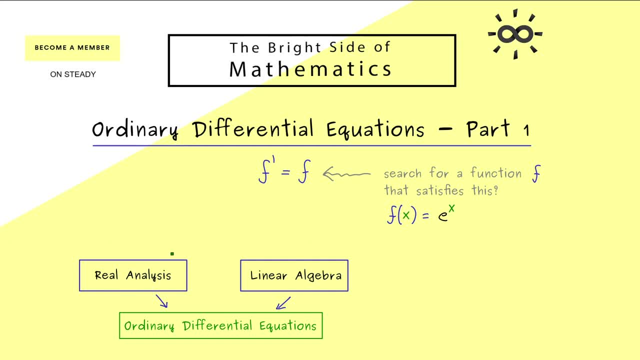 have video courses where you can watch the relevant parts. However, if you are very new to mathematics, I would like to suggest that you first watch my start learning mathematics course. There I tell you about typical notations: what numbers are, what sets are. so all the foundations. 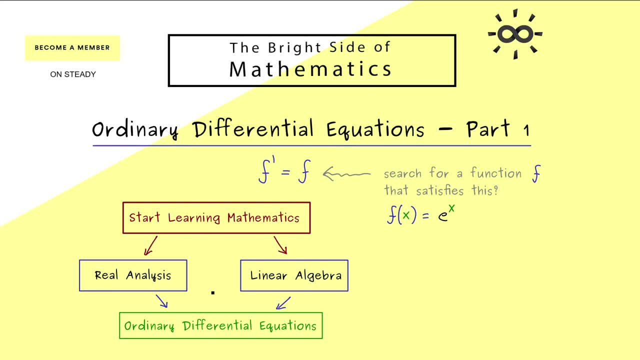 you need to understand the rest here. Okay, so now you know what we need and you see we don't need a lot of multivariable calculus, simply because we will not talk about partial differential equations. We will not consider partial derivatives in the equations, just ordinary derivatives. 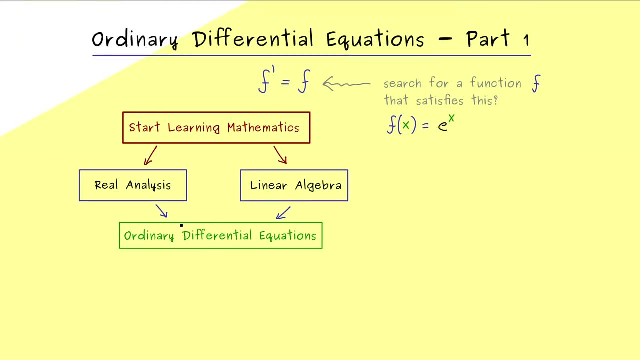 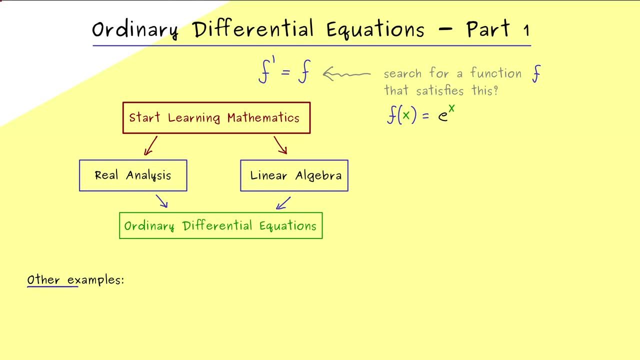 Indeed, this makes the whole topic much easier to deal with. However, in order to motivate you why ordinary differential equations are still interesting and very important, let's look at some other examples. For example, you might know that in physics, one use dots for denoting the time derivative. 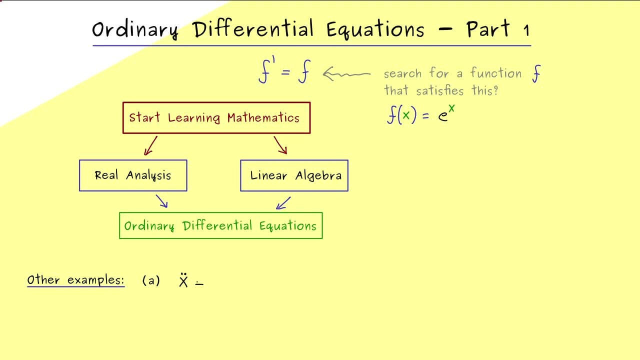 Hence this. This here is the second derivative of the function x, And now this should be equal to omega squared x. Indeed, in physics, this equation here describes a so called harmonic oscillator, And depending how much you want to calculate with complex numbers, you have a minus sign. 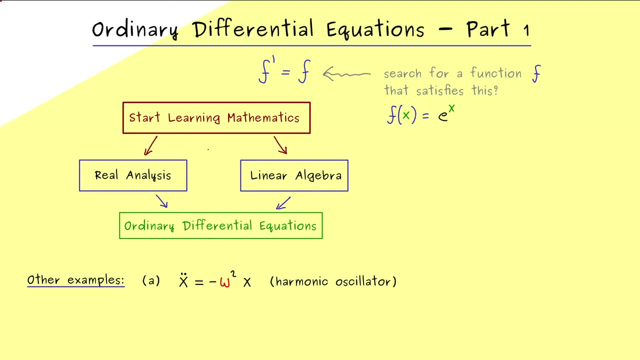 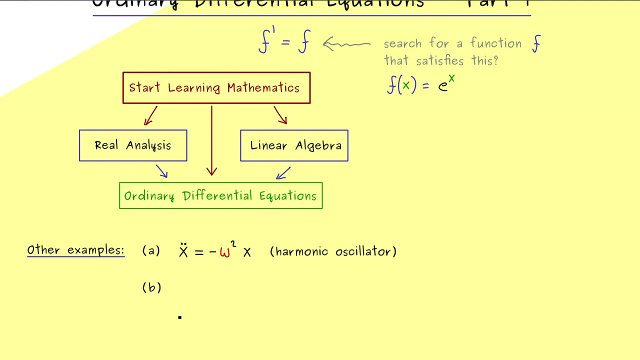 here or not, And there I should tell you: if you don't know complex numbers, you should check out my start learning mathematics series. However, in the end here, complex numbers will only be important for some calculations. Ok, so now we can consider another example, also given by physics. 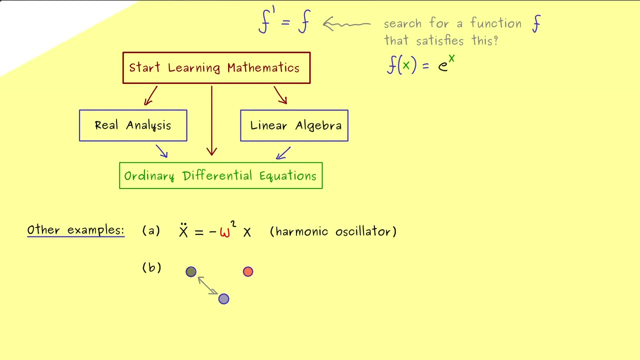 Indeed, this one is easy to explain. you just have three planets here and they will interact with gravity. So, simply said, they will attract each other. And now, if you describe the one planet in three dimensions, with a vector x and the,